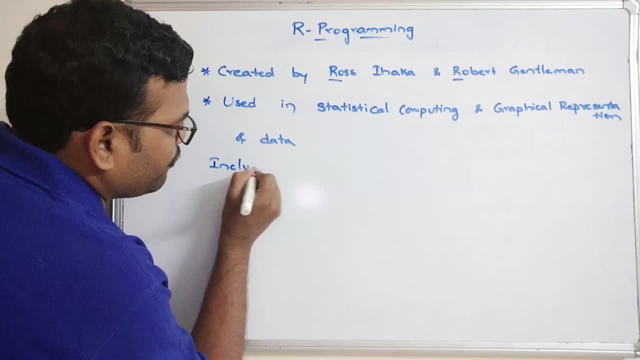 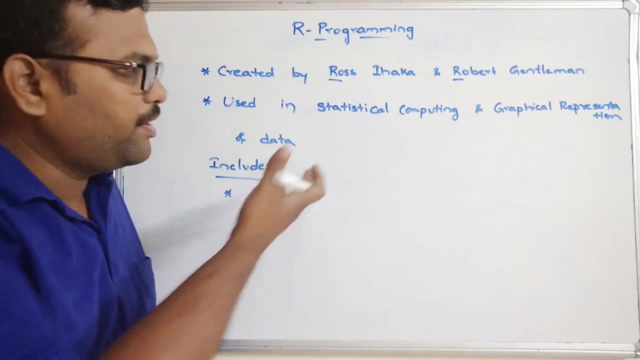 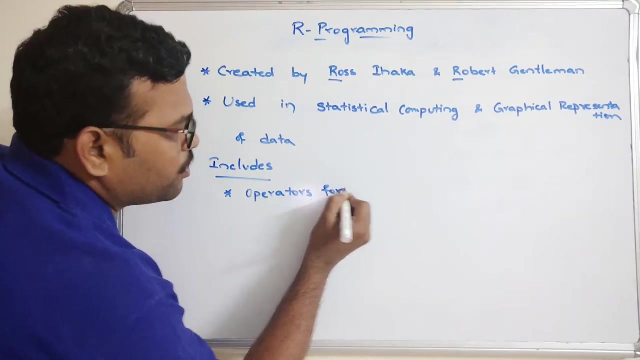 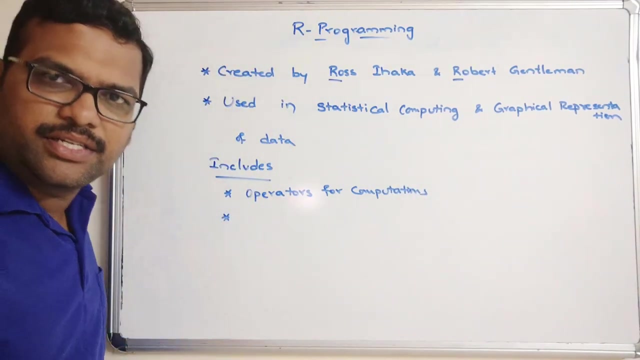 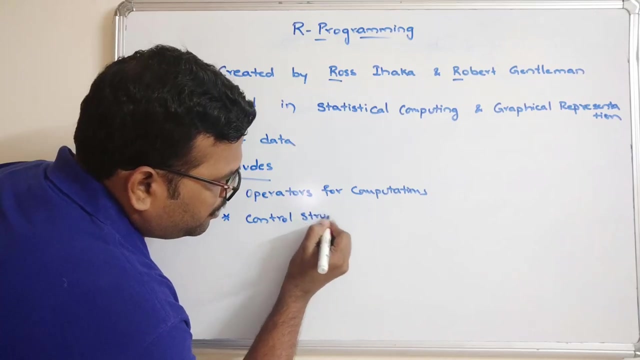 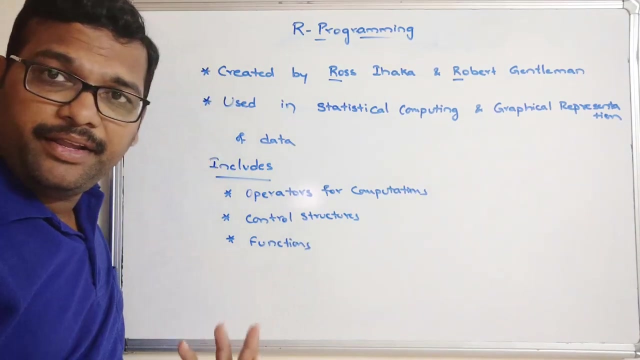 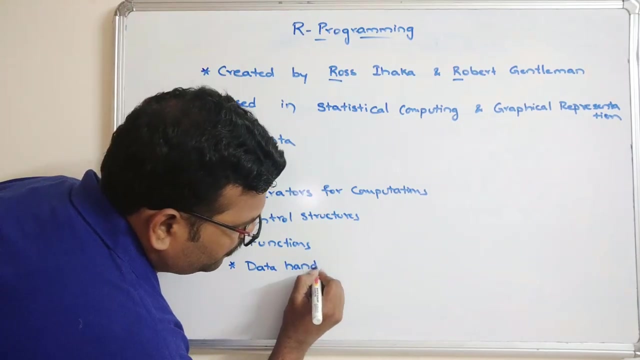 So what will be included? So R-Programming includes normal operators for different computations. So the first one is the operators for calculations or computations, And the control structures- right To say the flow of control- and functions to define the modularity and data handling techniques. 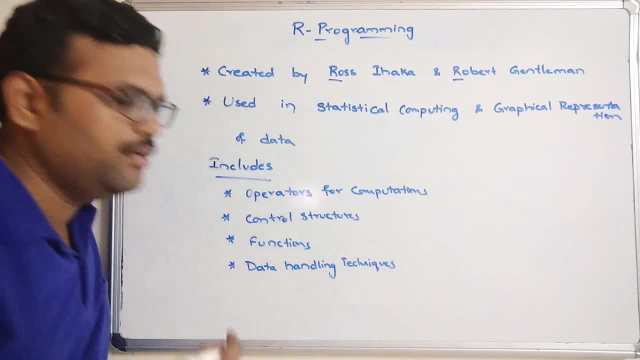 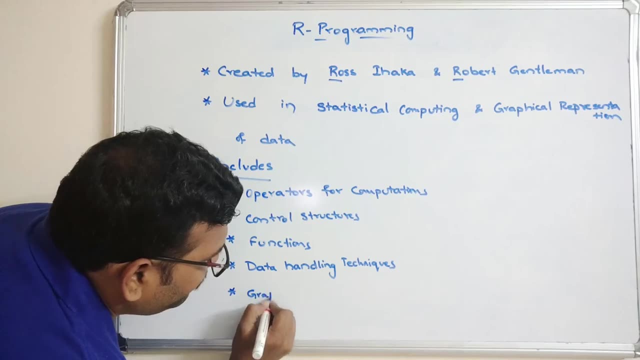 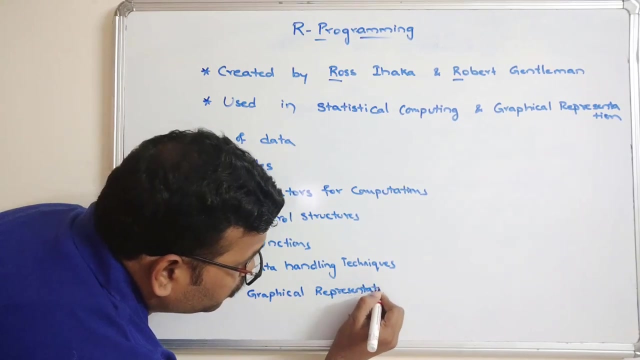 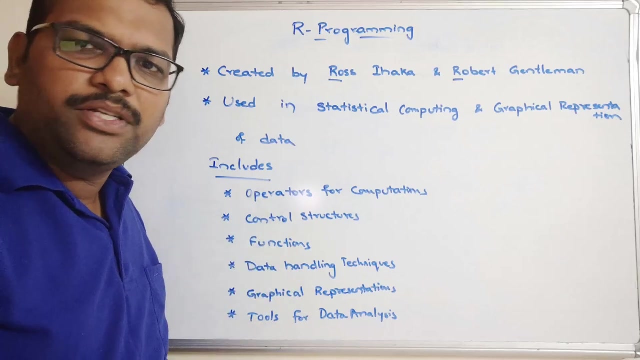 Data handling techniques. So there are a few techniques to handle the large amount of data, Okay, And graphical representation: Graphical representation. And also we will see a different tools for data analysis in order to analyze the data. So there are different tools available in this R-Programming. 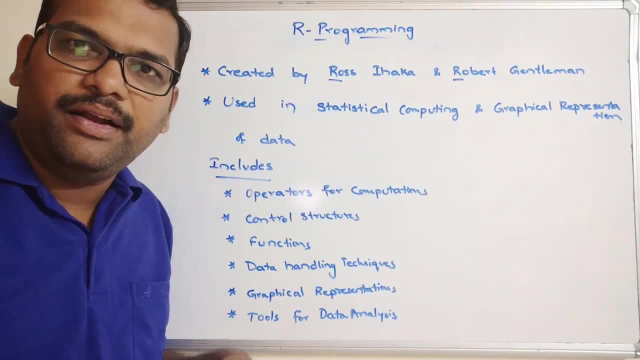 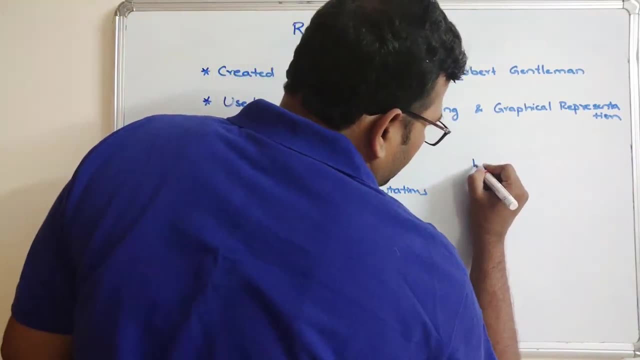 So we are going to see those tools for a different data analysis, Right? So these are all tools, So all things will be included in our R-Programming. And now we will see the features, some of the features of R-Programming. 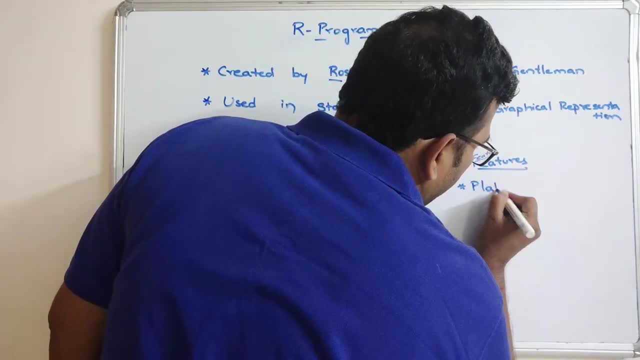 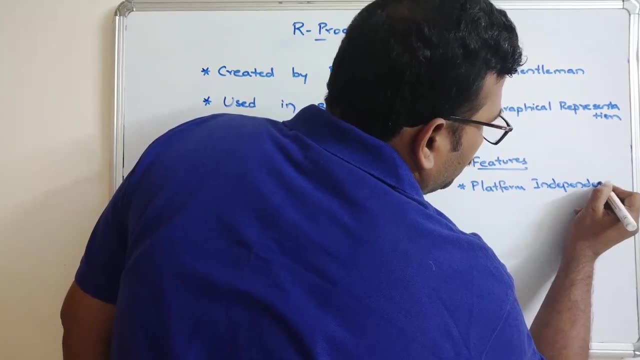 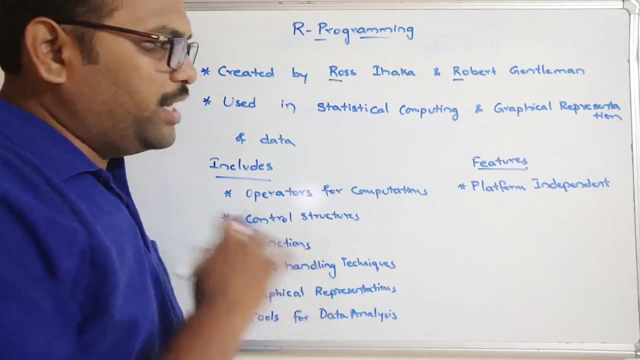 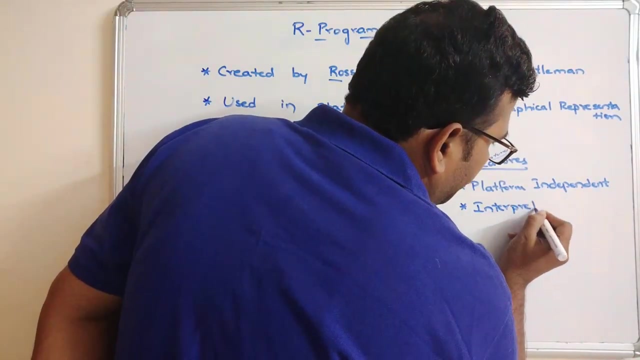 So the first one is a platform independent. So that means once you write the code, that can be run on any type of platforms, right? So that is a platform independent. So, And the next one is an interpretive code. So interpretive allows the user to use the code and the user can see the code that is. 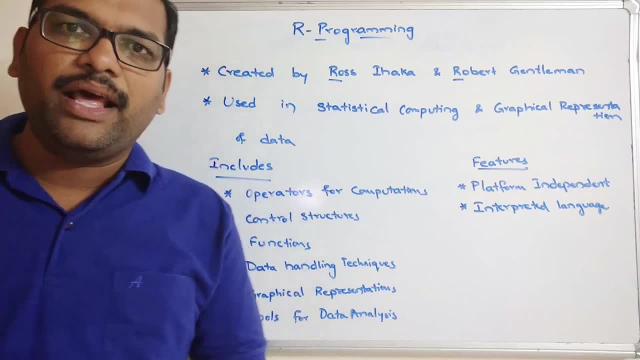 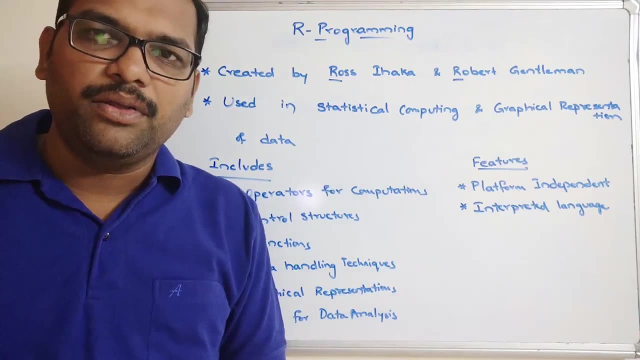 being running on the platform. So interpretive language- this is also the most important Interpretive language. So interpreted language means there is no need of compilation, So directly the programs will be interpreted. So instruction by instructions will be get converted into the machine language. 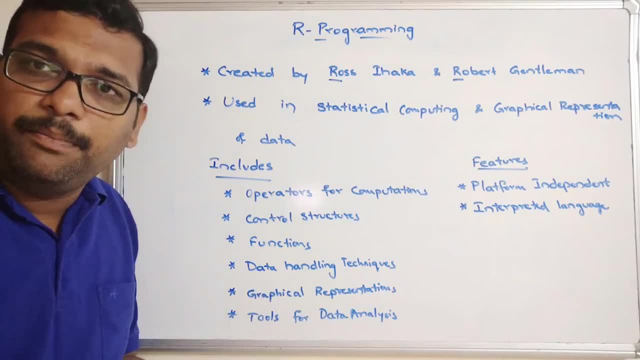 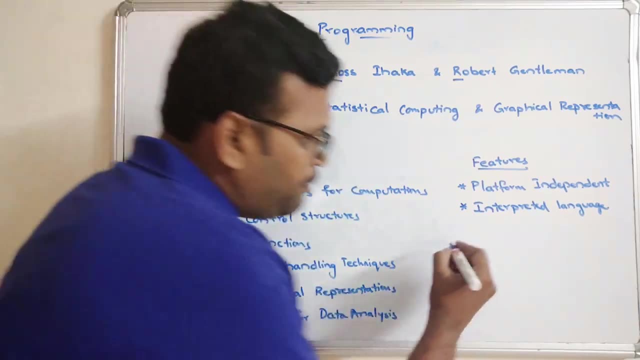 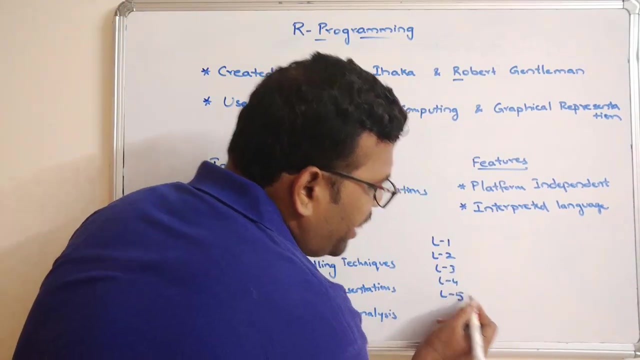 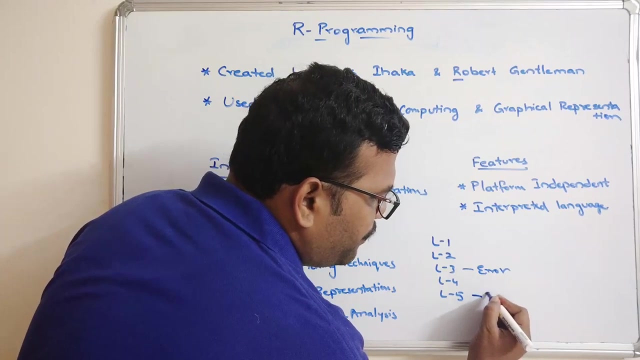 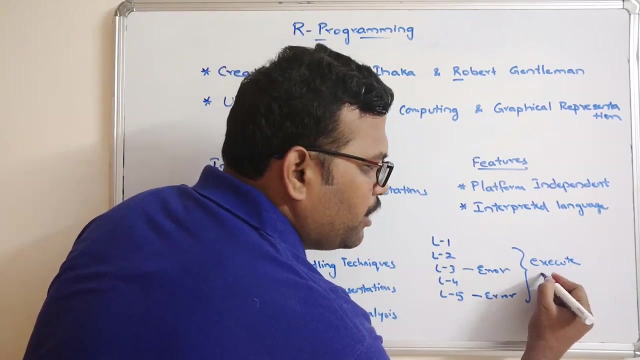 So example: Python is also an interpreted language Similar to that. this R-Programming is also an interpreted language. That means So if a program is having some 5 lines- L1, L2, L3, L4 and L5- and if you are having some errors in line 3 and line 5, so once you get executed, if you execute this program, you will get only one error. 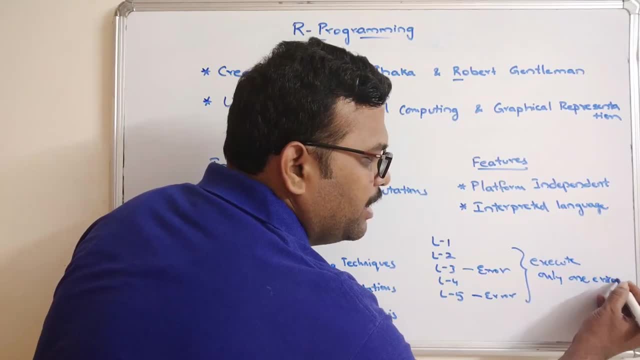 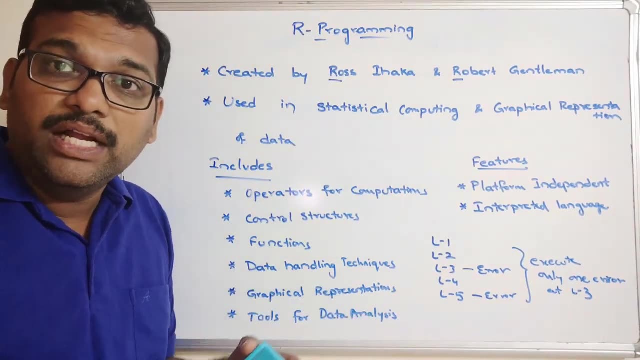 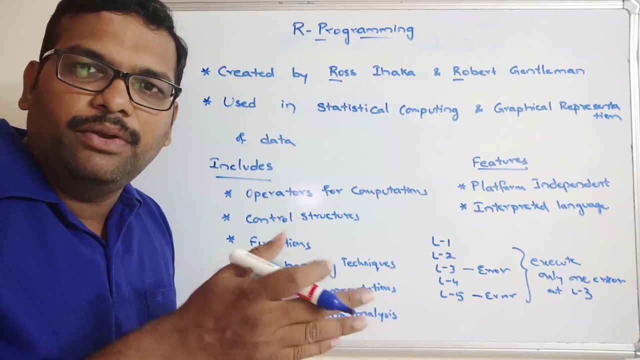 It doesn't show both the errors. right, It will show only one error at line 3.. It doesn't show both the errors because this is an interpreted language, though the transformation from high level language to the machine language will be done instruction by instruction. that means line by line. 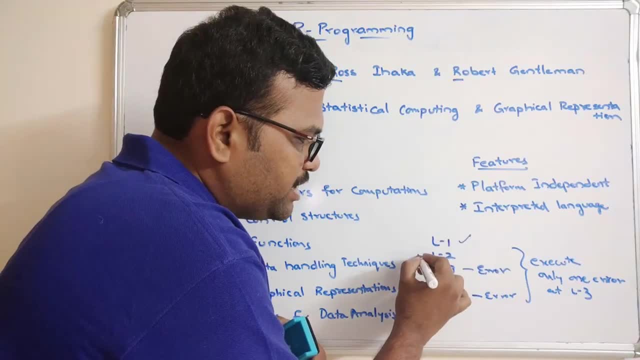 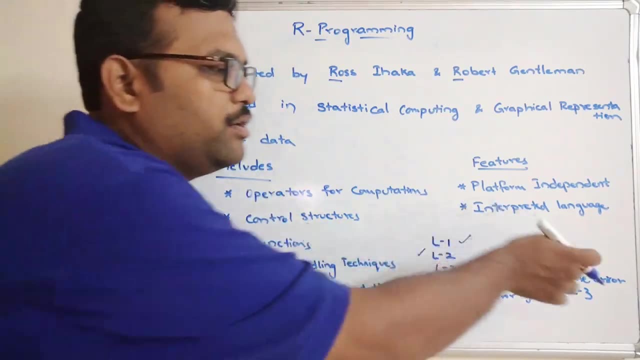 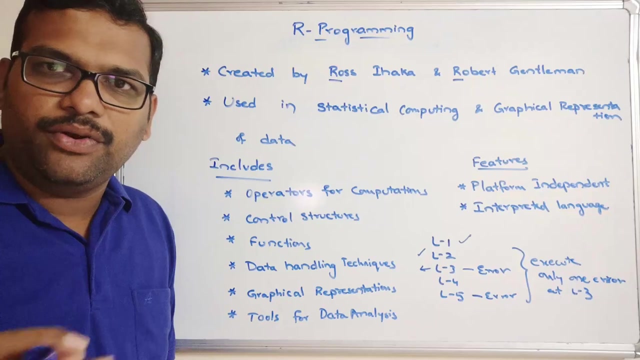 So where the first line will be get executed and immediately the second line will be get executed, and whenever the interpreter try to execute this line 3, it will get an error and it will raise an error. So until this error has been solved, the L4 will not be get executed. that means the line 4 will not be get executed. 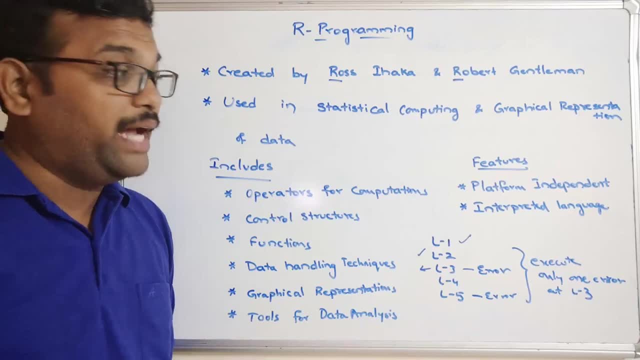 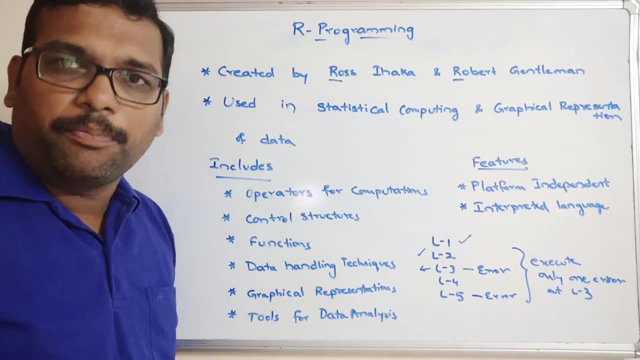 So at a time we will get only one error, So that we call it as a interpreted right. So here also, we are going to write the program and we are going to execute the program, but the conversion will be done by using a line by line right. 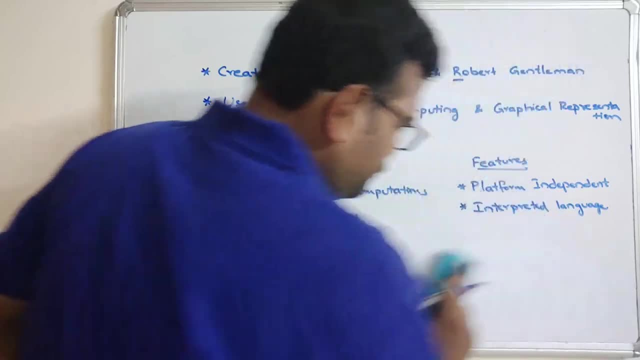 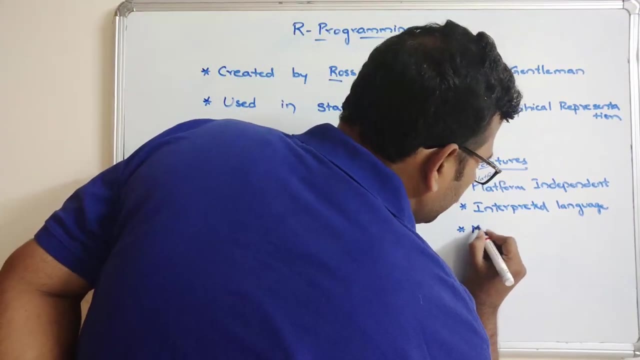 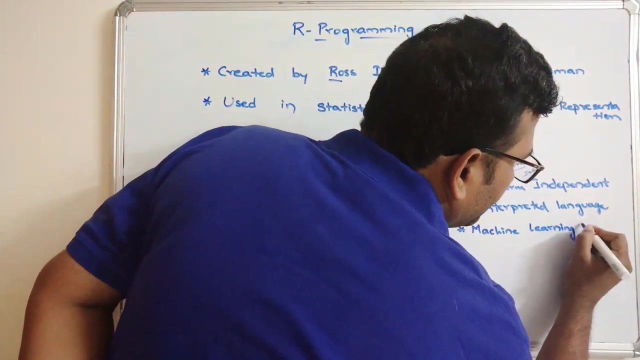 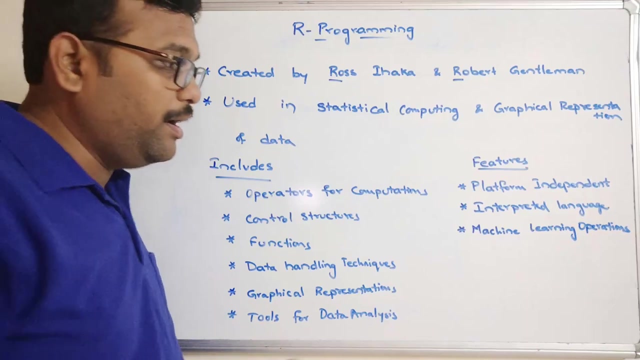 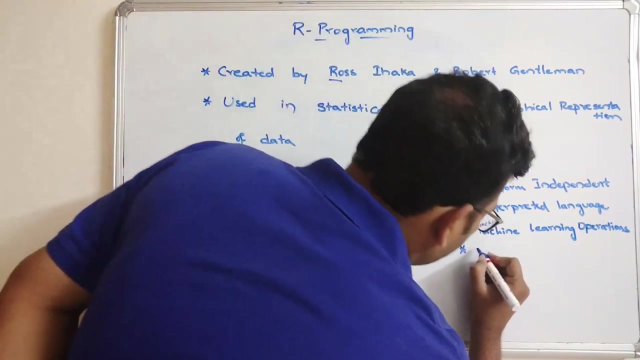 So that is one more feature, And this is most suitable for implementing the machine learning operations. So suitable for implementing machine learning operations, Machine learning operations right, And also this R programming, is having a wide variety of packages. Large number of packages are available. 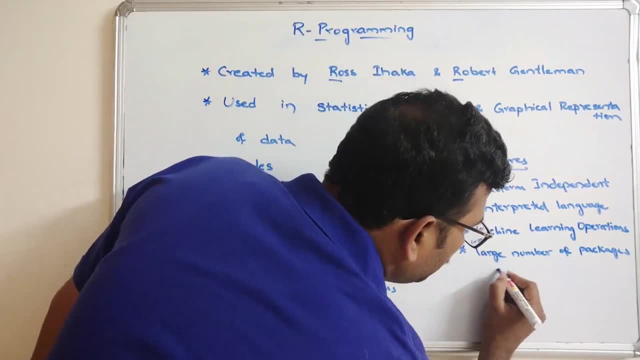 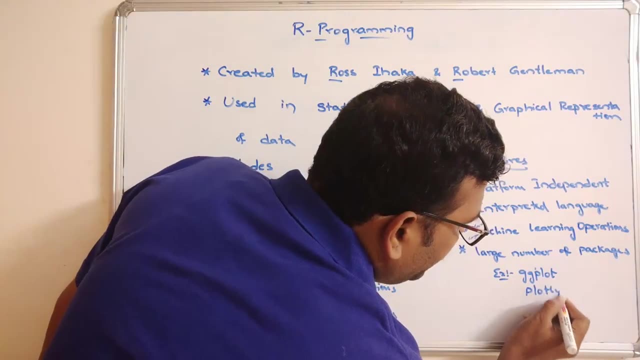 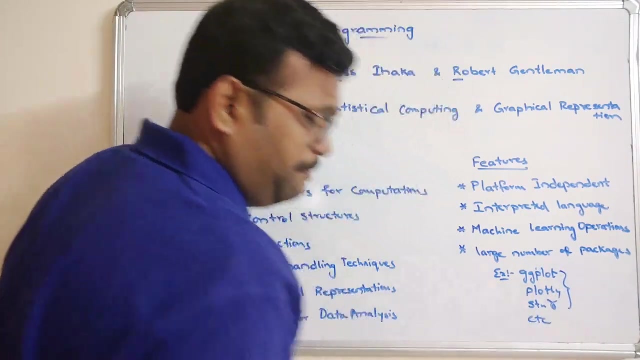 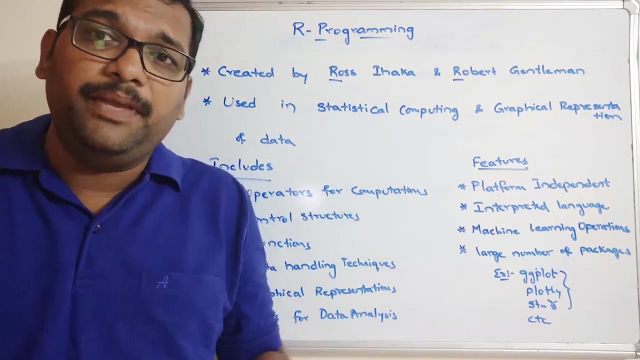 Large number of packages are available. For Example, there are some packages like DG, plot plotly right, So some string R. So those are all basic packages. So R programming, R programming, that means only the default packages will be available once you open the.